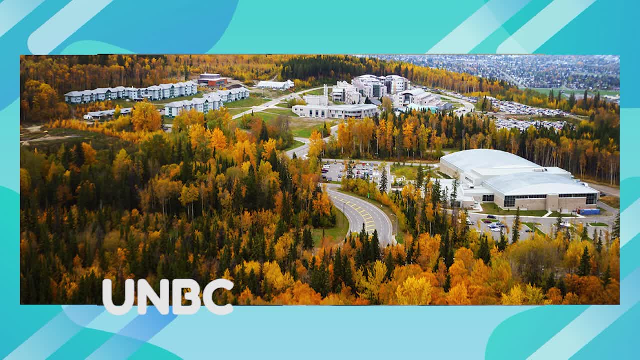 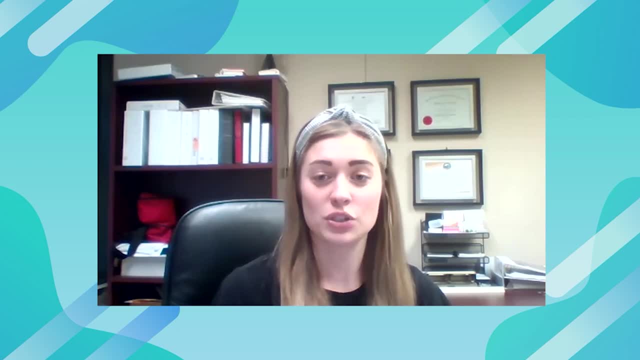 the environmental engineering program at UNBC and UBC. It's a joint program. I graduated in December of 2017 and then I decided to do a little graduation trip around the world, which I do recommend everyone does after they graduate, just to make sure you travel before you get a job. 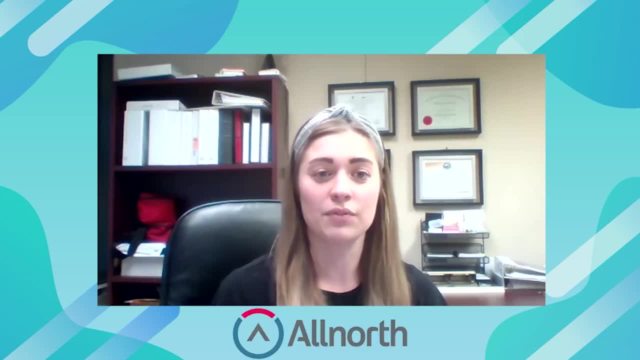 And then I was able to come back and get a job with All North in April of 2018.. So I started as a civil engineer in training. I did that job for about a year and then I changed over to management. So I started as our construction services coordinator. I did that for about four months. 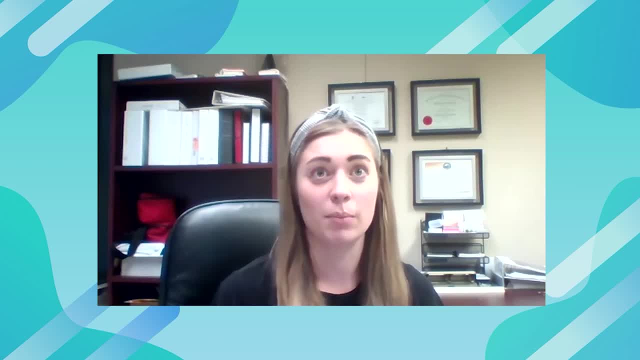 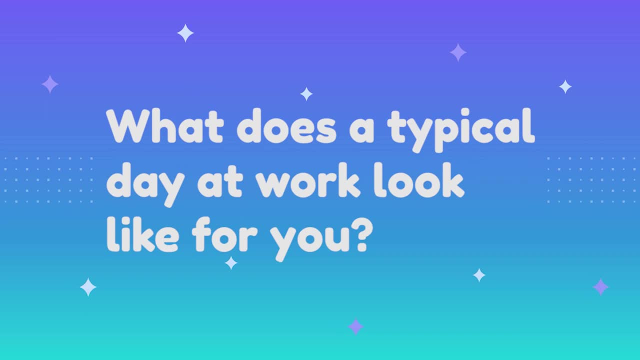 and then I was pushed to construction services manager. So I've been that for about almost two years now. You mentioned that you kind of work as a consultant. now Could you just give us a little bit more detail of how your day is like? For sure, 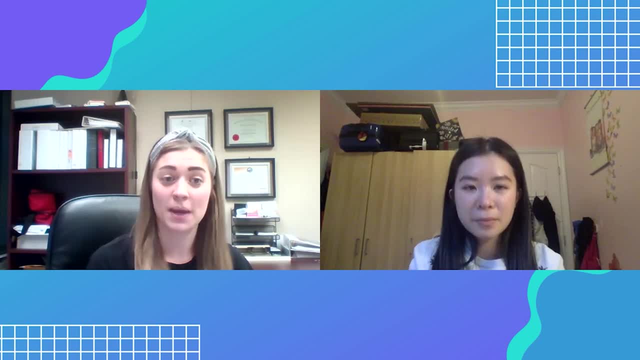 yeah. So obviously in consulting engineering it's very project dependent. It's very dependent on what's kind of going on with the projects in northern BC and what All North is bidding on, what we're winning. So I'd say the most typical things I do are project management, So I do run. 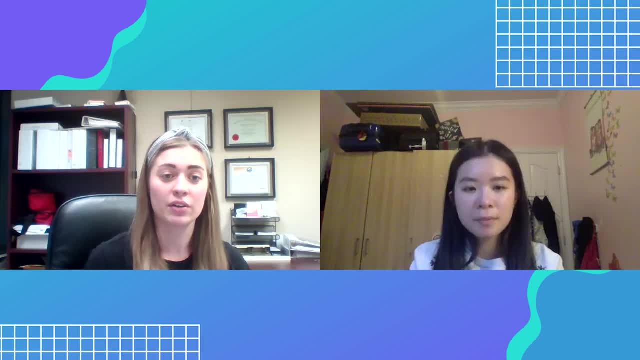 budgeting for our office. I run our lab that we have here on site. I'm our radiation safety officer, So I'm involved a large part in the safety program here And, yeah, a lot of training with our summer students and our new hires So recently. so we bid a lot of work with the. 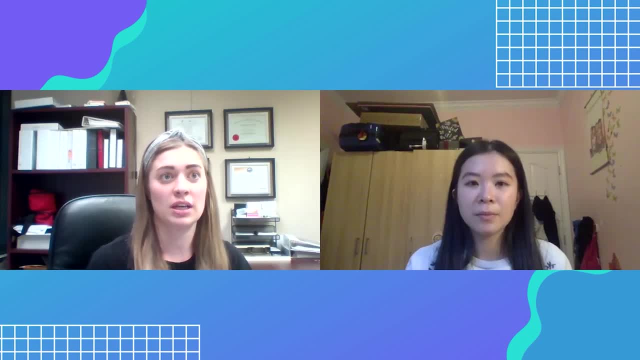 Ministry of Transportation. So the Ministry of Transportation creates new roads and bridges around the province. So a lot of the time I will be the project manager for All North because they are contracted out by the ministry to do quality construction. So I'm a project manager for All North. 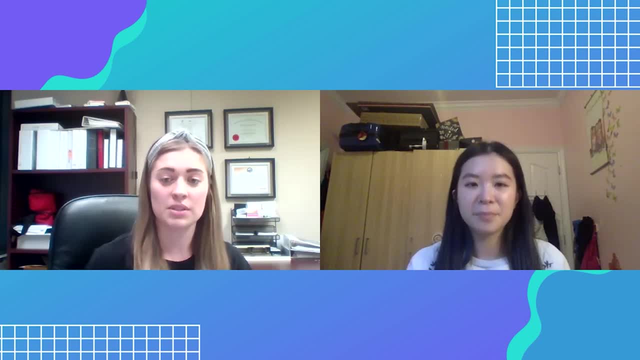 So basically, I'll be in charge of sending people to site and making sure that they are following the technical specifications for the project. They're doing the quality management checklist, making sure everything conforms to the ministry's standards and codes- Awesome, It sounds like a lot of responsibilities as well. 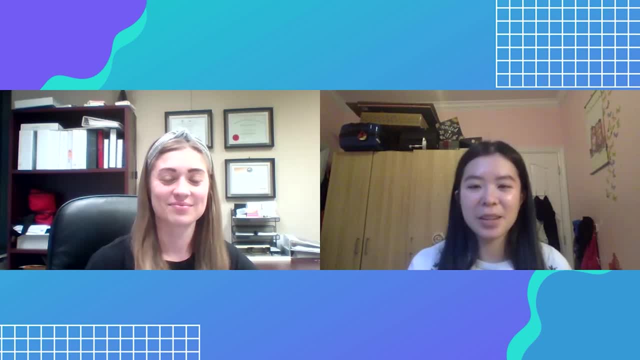 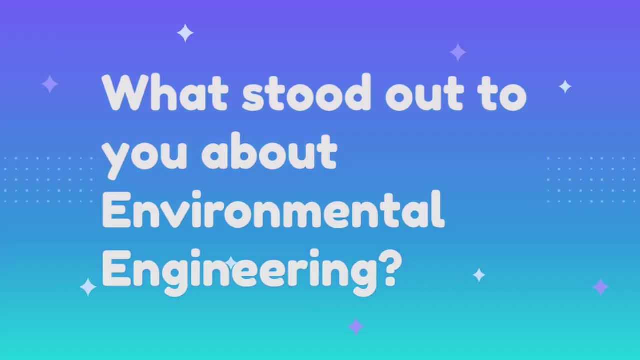 Yes, Yeah. Moving on to the next question, You mentioned that you really like engineering from a really young age. Could you tell us what stood out to you about environmental engineering specifically, And can you tell us a little bit about what you do? 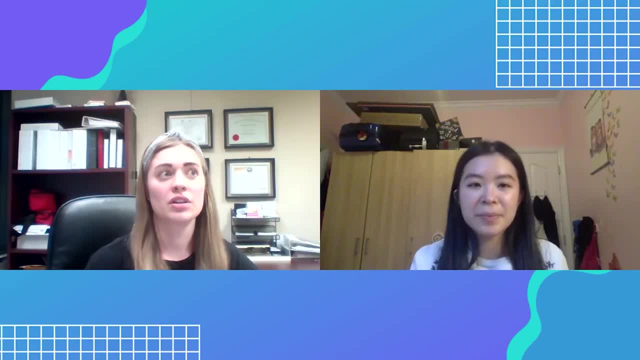 Can you tell us, kind of, why you decided on pursuing it? Sure, Yeah, So I think, like I said, math was always my strong suit. Highest grades were more so in math. So I knew that I wanted to kind of go into something math related And engineering kind. 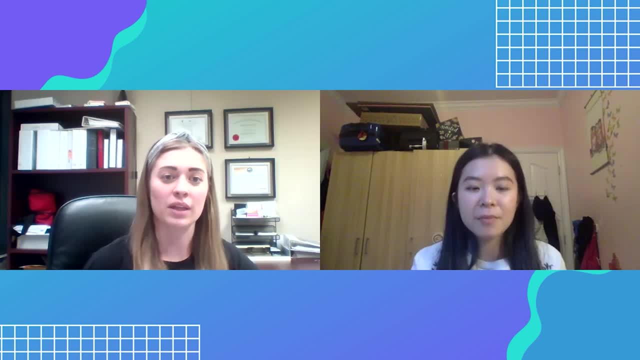 of just ties in the practical aspect of math. I found Like it's not just straight mathematics but I also get to learn how that math works and then how I can apply it to real world situations. So that's something I've always been super interested in, is kind of making a difference. 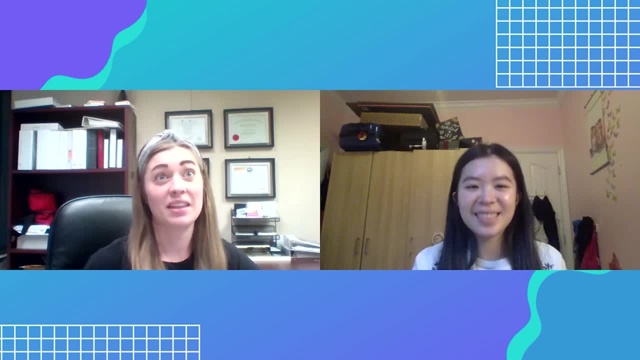 And I figured engineering would be a good way to do that. And then the environmental portion. like I said, I always knew I wanted to do environmental, just because I love being outside, I love working in the outdoors. I do aspire to go into renewable. 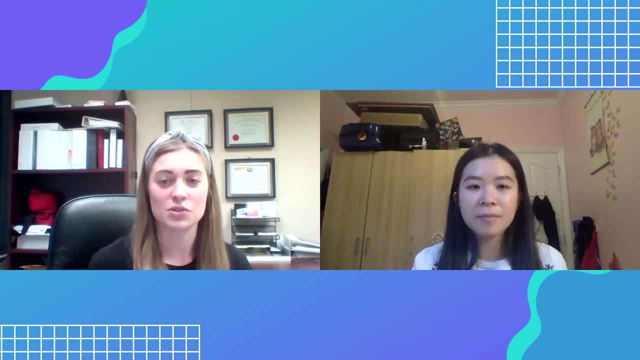 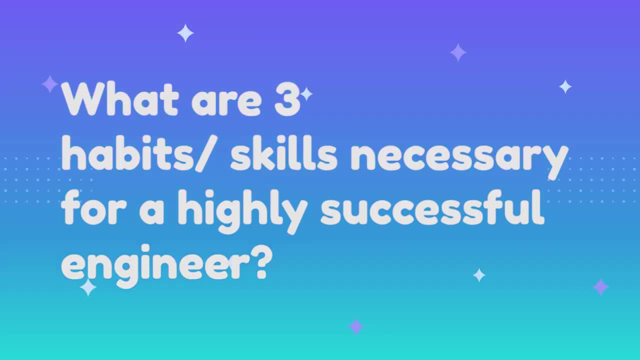 energy one day. So I figured that environmental would be the best stepping stone for that. So that's why I chose that program- Awesome. Next question: What are three habits or skills necessarily for highly successful engineers? I think one of the big things is: you have to be. 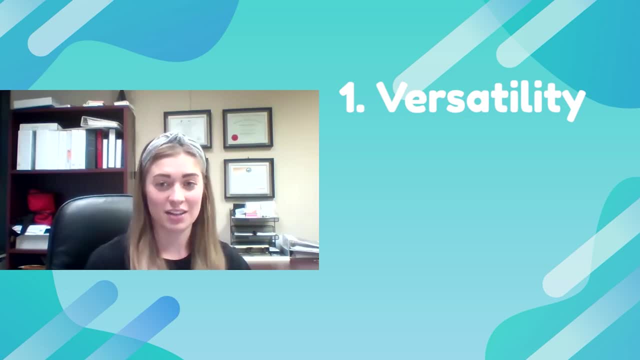 very versatile as an engineer, especially in consulting. Like I said, there's so many different things going on And I think that's one of the things that I've been really interested in is being able to do, And I think that's one of the things that I've been really interested in- is. 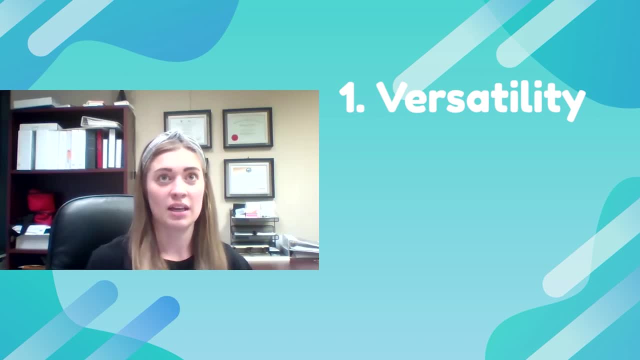 being able to do, And I think that's one of the things that I've been really interested in is being able to do, And I think that's one of the things that I've been really interested in is kind of have to be able to do a bunch of different things. The second one, tying on to that, would be: 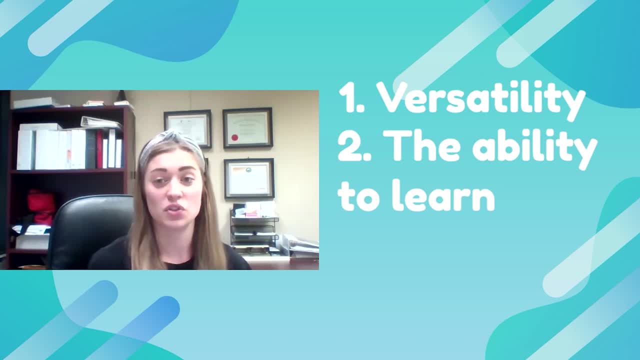 the ability to learn how to do different things, And I believe that engineering school really teaches you that there's just so much going on all the time, And school, more so, teaches you how to learn. It doesn't. it's not the same as your job. It's never going to be the exact same, but 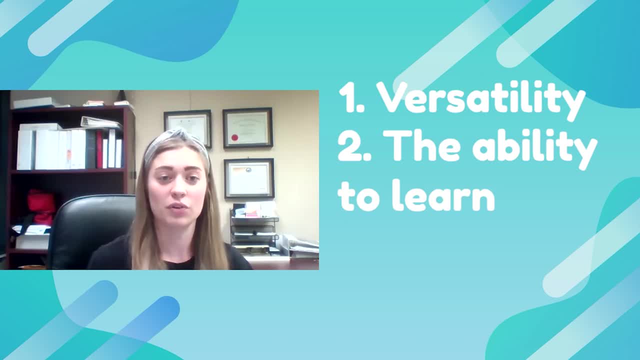 it teaches you how to actually learn. So when you get kind of into the workforce you have the ability to learn how to learn, if that makes sense. The third one I want to say is probably time management. Being an engineer with a lot of different things going on, especially in the 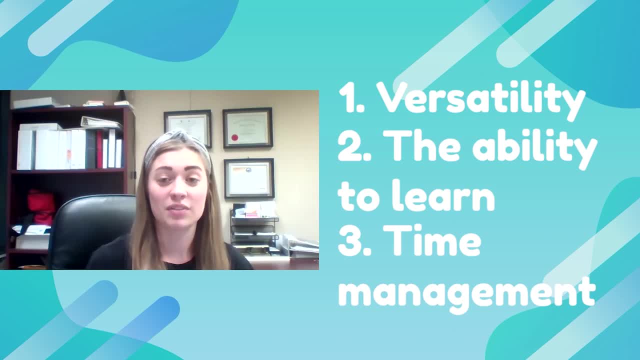 consulting world. you need to learn how to manage your time effectively and just make sure that you kind of are able to prioritize your tasks and you're able to still book off time for non-work purposes as well, because it's very easy to get consumed and work and make that your entire life. 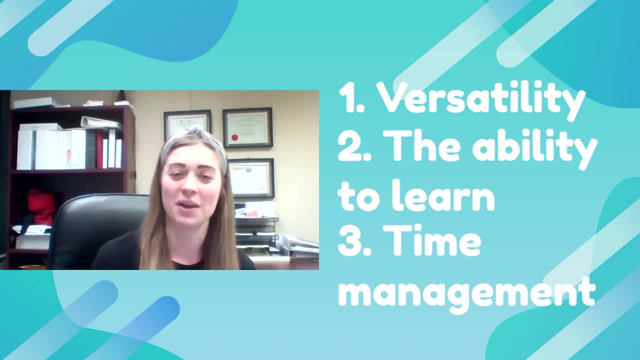 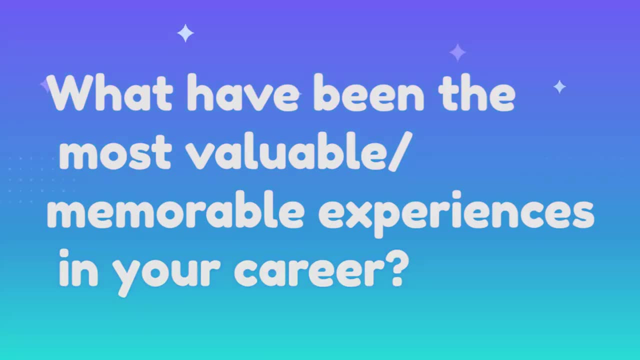 but I do believe it's important to make sure you have time for fun as well. Yeah for sure. it's always good to have a work-life balance. Yeah for sure. So, moving on to the next question: what has been some of the most valuable or most memorable events that has happened over the course of your 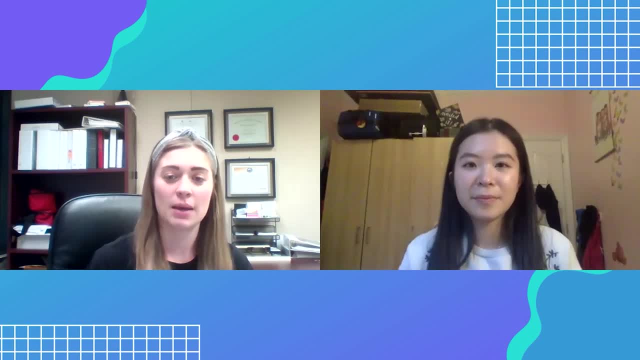 career. One of the most valuable things for me has been the support that I have from Olmert and kind of the support I have from my superiors. Like I mentioned, I was a civil engineer in training for under a year and then I was very quickly pushed into a management position and I was scared. I was 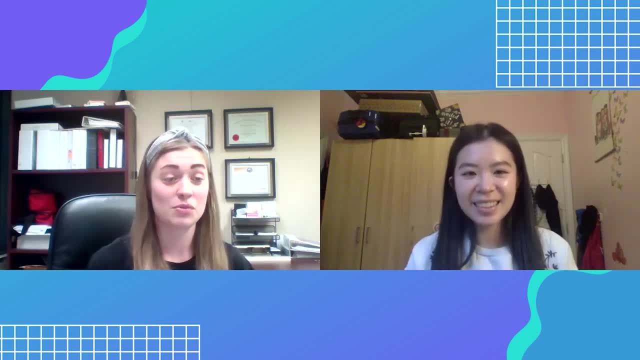 nervous. I didn't think I could do it, but I was able to do it. and I was able to do it Because I was still a recent grad- I was just fresh out of school- but because of the support that I had from my superiors and them being like: no, you can do it, you are capable of doing this. 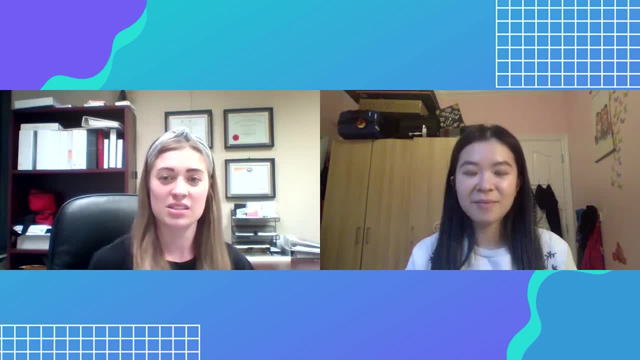 you are competent enough, you are good enough, and just kind of having that support and that transition phase between the EIT position to the manager position was so helpful and like it's something that I'll take with me for the rest of my life. Next question: what were some of the 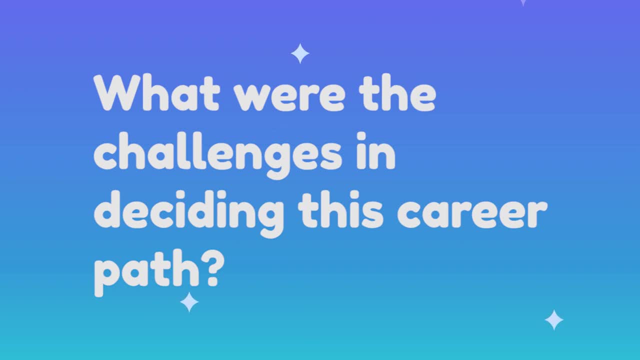 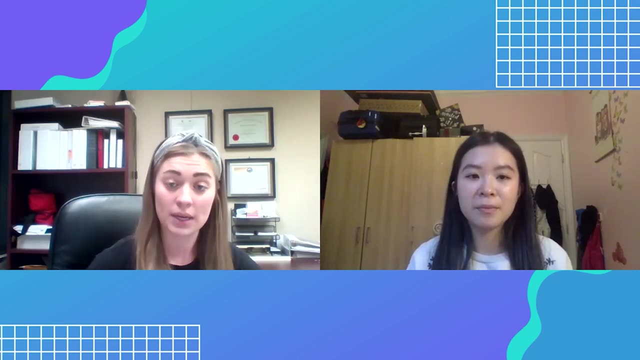 challenges in deciding a career path. Did your goals or plans change during your studies or once you had started your career In engineering? there's kind of two routes you can take. You can take the project management side or you can take the design engineer side, and the world needs both of them, so there's no wrong. 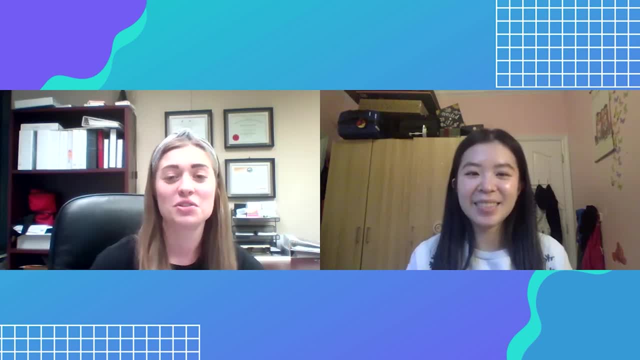 answer in the way to go. I always kind of knew that I wanted to do the project management side, so I was lucky that that opportunity presented itself. When I was in EIT I was mostly all out in the field, so I was doing a lot of materials technician work. I was a survey assistant. 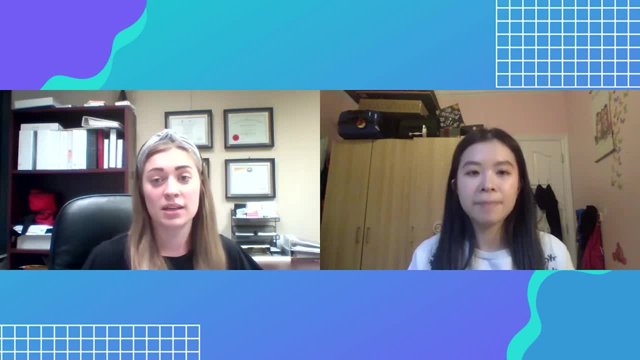 I was doing quality control work. so I was working at a mine site actually where I was being the quality control manager for all the construction going on. so it was very heavily field-based and I would not change that for the world because I learned so much being out in the field and I 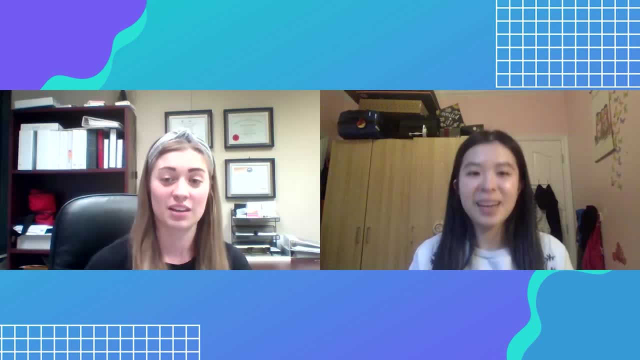 believe it's very important for engineers to start out in the field so they can have an understanding of what goes on out there and in real world conditions and then bring it back kind of that understanding to the office. So I was lucky that my transition from the field to the office was 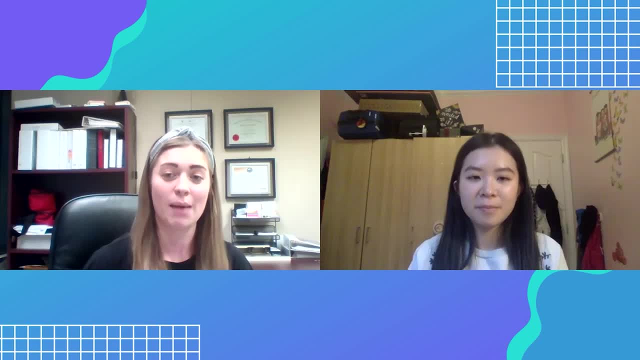 pretty seamless because I was able to understand the work that I was doing and I was able to understand what happened on those projects and then try and manage them. so I kind of had that overarching understanding of the project Transitioning into the school focused questions. 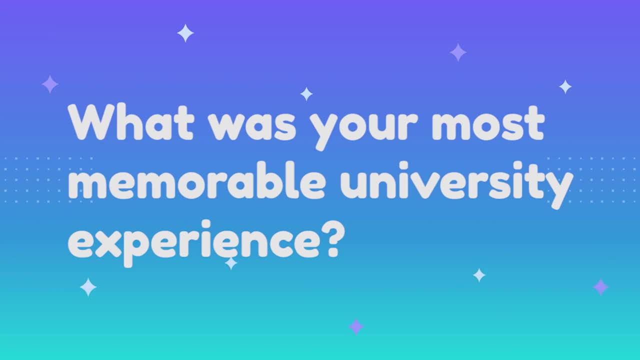 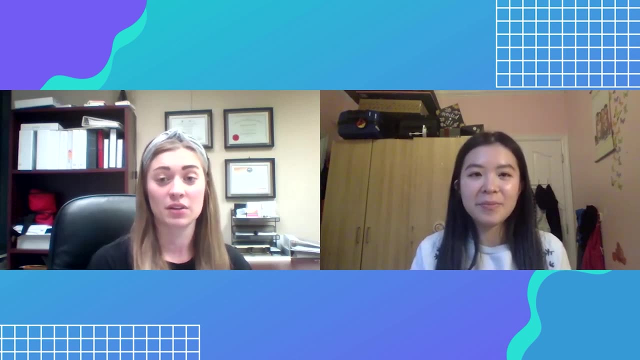 what was your most memorable university experiences, and if you could give tell us a little bit more about UNBC, that would be great as well. Most memorable university experiences had nothing to do with school. I was fortunate enough to play on the varsity women's soccer team up here at UNBC. 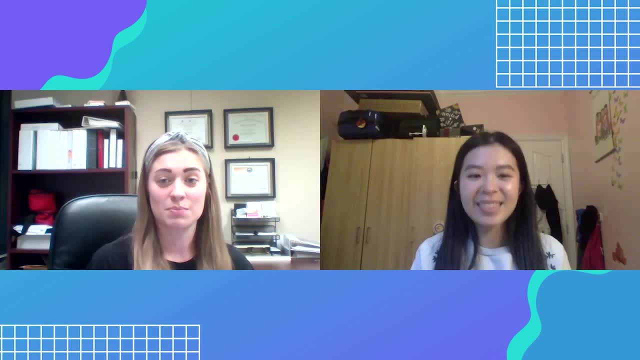 so I would say the best part of my university experience is that I had the opportunity to do a degree, was being able to to play a sport that i love while going to school and getting to meet so many new people and friends up here, and that's one of the reasons why i decided to to stay in. 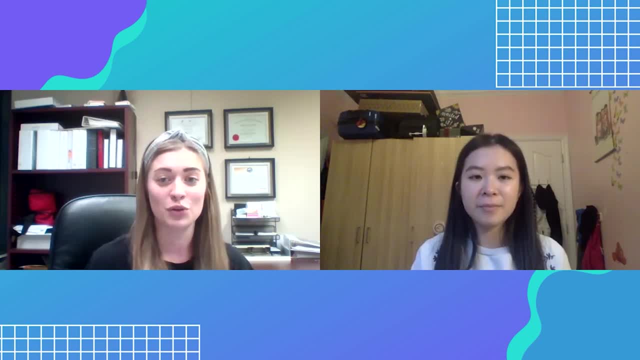 prince george after i graduated because, as i mentioned, i'm from vancouver, so i was a big town girl and i've now moved to the small town and i wouldn't change it for the world. so umbc is amazing. um, it's a, it's a really small university, but it's very new, very modern, very innovative. 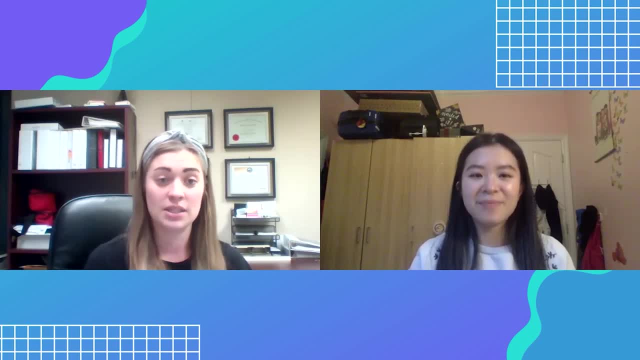 i loved being able to do both um, unbc and ubc because they're such different experiences, right. so when i first moved to umbc, i didn't know anyone. i was coming up brand new, just fresh out of high school, but i was able to meet friends very easily. one because of the soccer team. 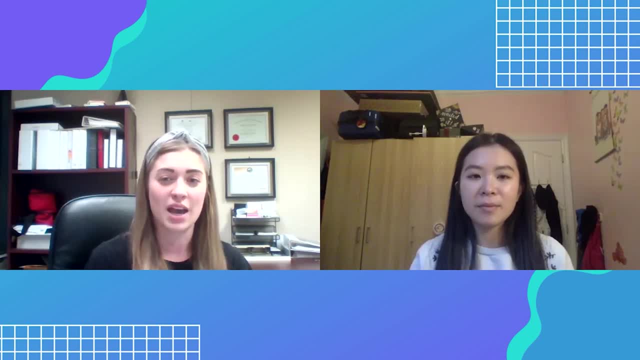 and two because umbc is such a small town feel, so it's a really like close, tight-knit family kind of feel and i really enjoyed that because it was way easier to meet friends, like everyone up here is so friendly, so welcoming, just like happy to have you here. so i would recommend you mbc. 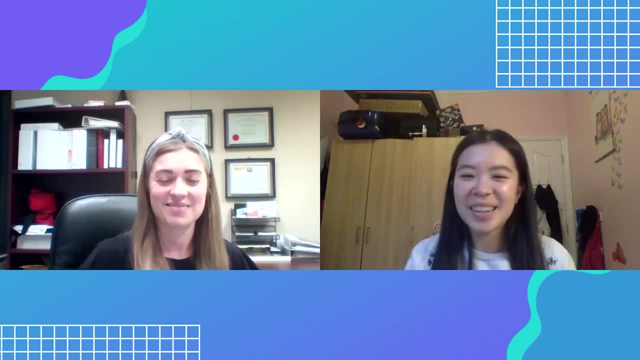 to anyone. i loved my experience there. so the next question is: if you could do one piece of advice to your younger self, what would it be? i think one thing that i would tell myself going through school again is have more fun, because i, like i mentioned, i played soccer and i was very 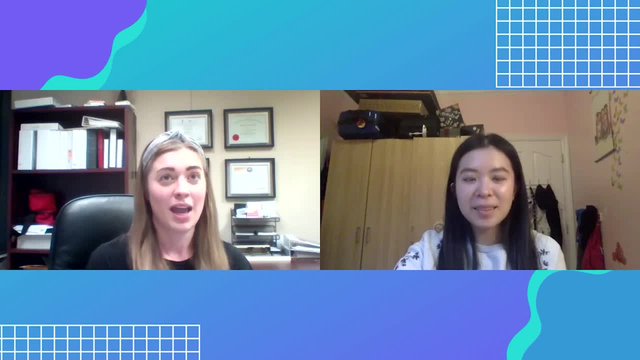 academically driven, so i always wanted to do well in school, and trying to balance soccer school and a social life is very important to a college student and them, and when they go to school and they're out there, they're there on their own and they, Jeanine, I love you. source.